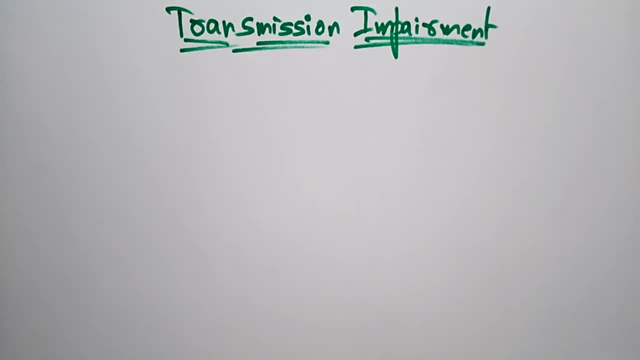 vary. okay, so if I pronounce like good it will be, Listen by you, like would like, that means some disturbances will be there. the word, whatever I am saying, the center, the receiver, you are the receiver, you are receiving, maybe differentiate, Okay, you can't. Maybe you may not receive the exact information. whatever I'm sending. that is a transmission impairment, So it's nothing but. 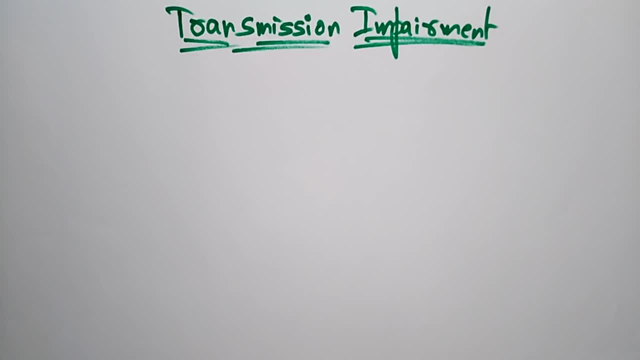 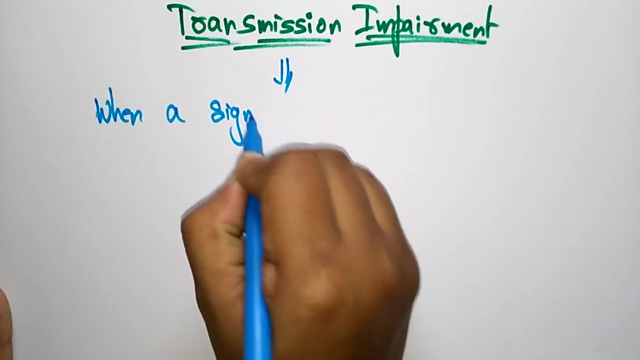 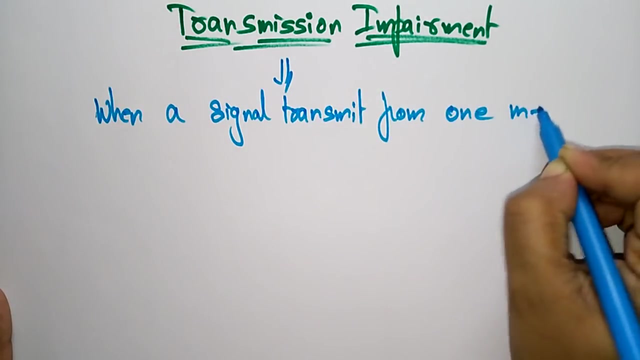 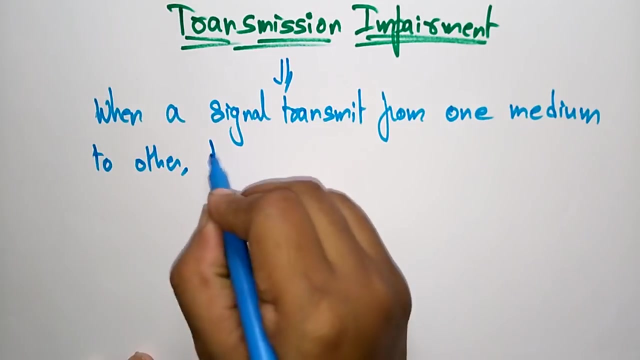 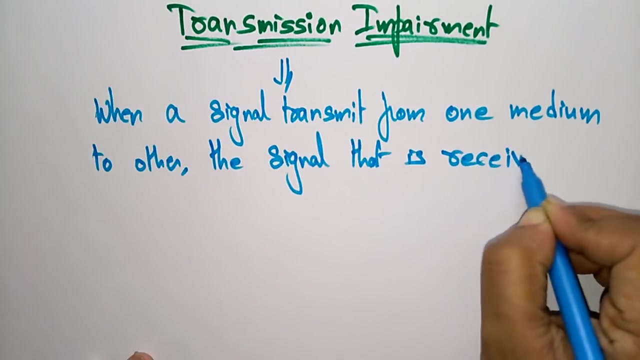 the receiver may not receive the information, whatever the sender may sending, due to some various impairment that you call it as transmission impairments. let me write the definition: when a signal transmit from one medium to another, one medium to other, the signal that is received. the signal that is received may differ from may differ. 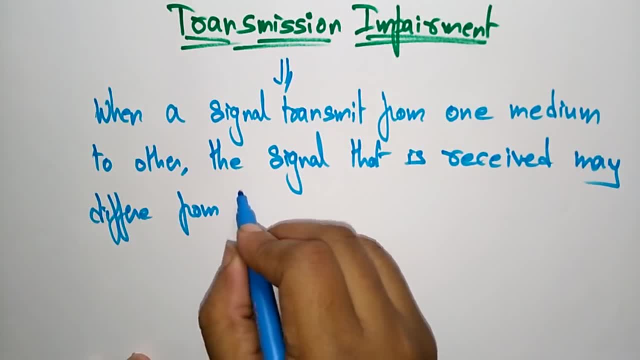 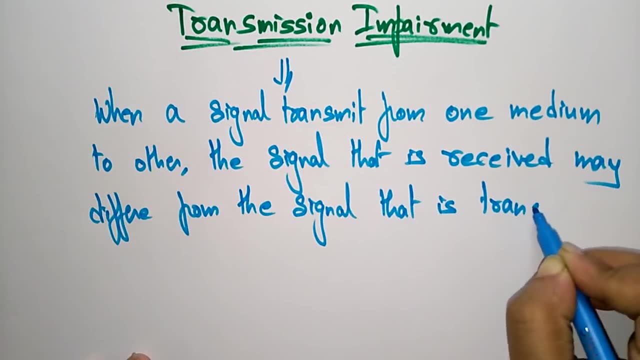 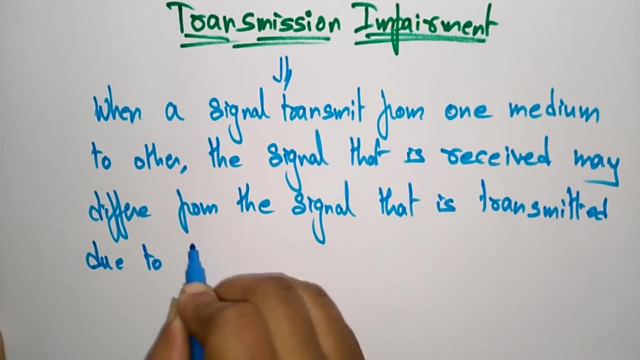 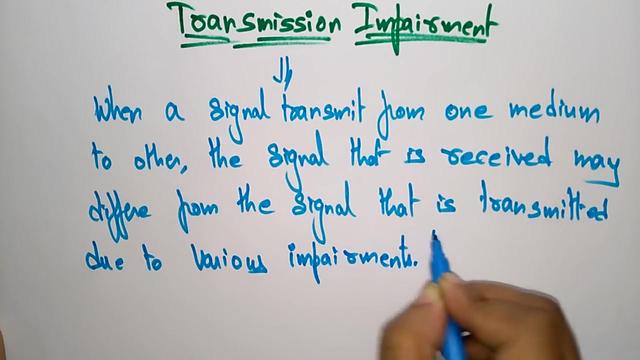 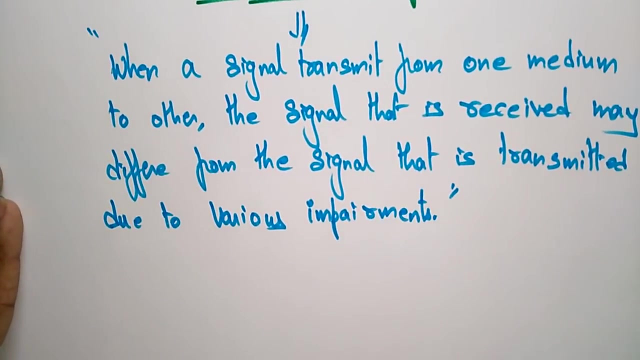 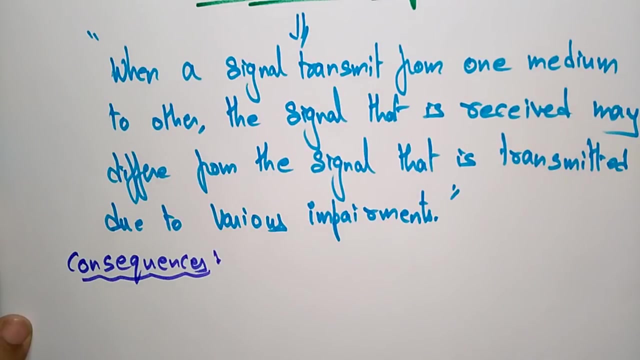 from the signal that is transmitted. the signal that is transmitted due to some various impairments, due to various impairments that you call it as a transmission impairment. so what are the consequences that are present in the signals? let's see the consequence. of consequence, if you take the analog signal, let's take for analog. 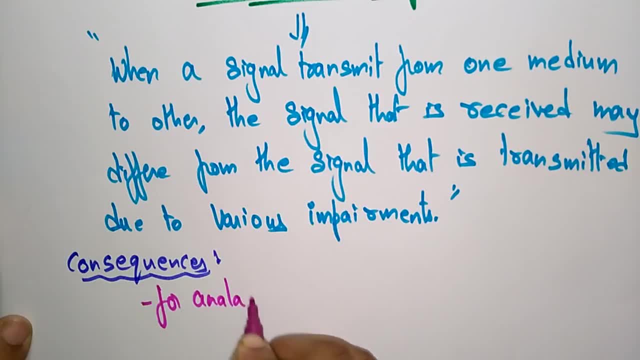 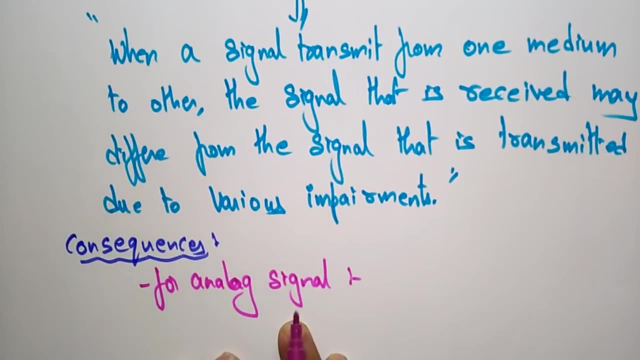 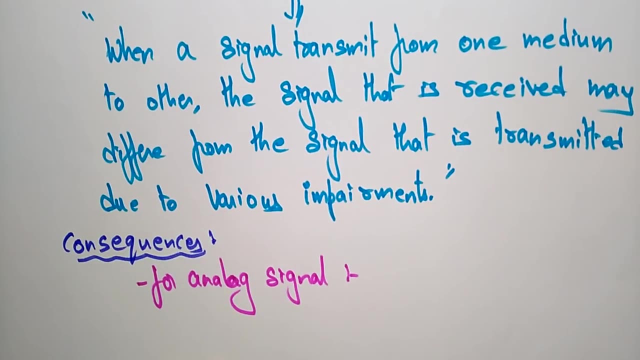 signals. what are the consequences? you will have came across analog signal. what are the consequences? you will have came across analog signal. so, in and if you take the analog signal, the degradation of signal quality, the transmission impairment is nothing. but whatever the analog signal you are sending from sender to the receiver, the receiver may receive the data in the form of degradation of. 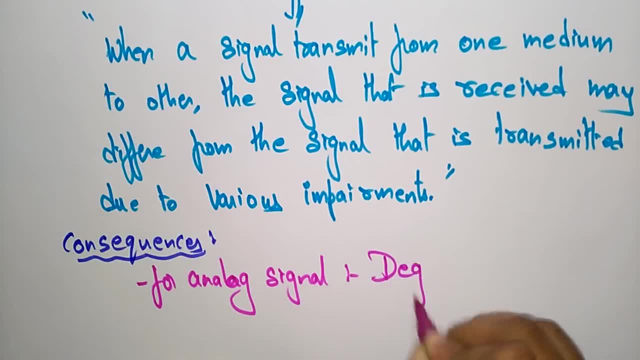 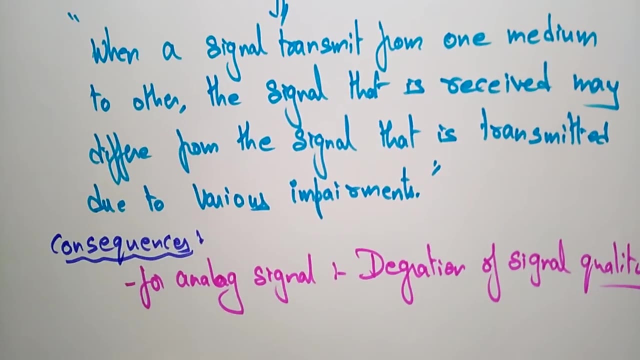 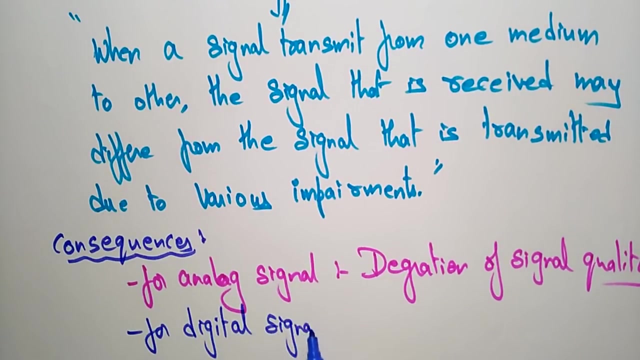 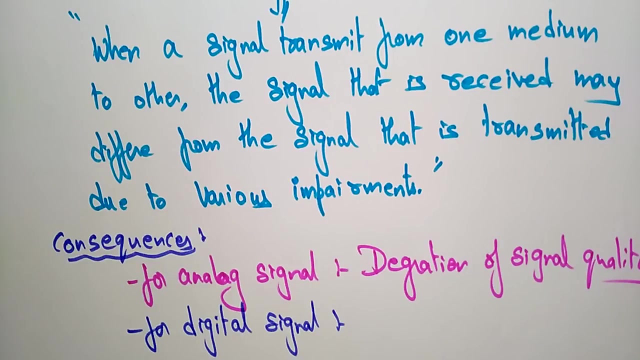 signal quality, degradation of signal quality. the receiver may not receive the exact quality of information. so that is a consequence. so next, if you take uh digital signals, let us take for digital signal. what is the consequence? so for digital signal, uh, digital means it's a numbers, that is, ones and zeros. in the form of ones and zeros, the bit may become error, the receiver may. 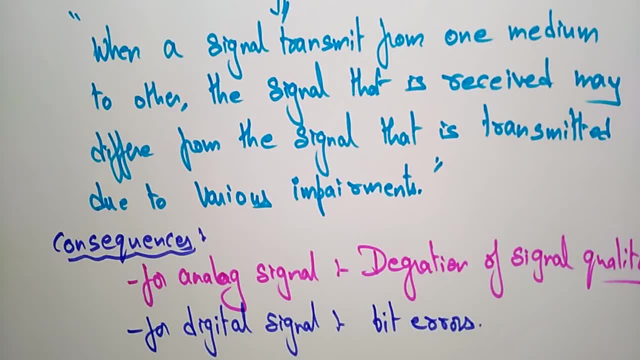 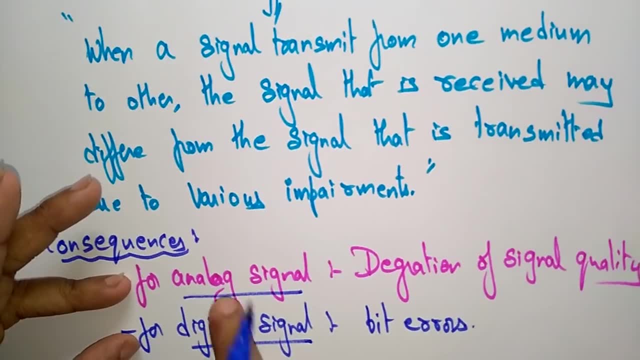 receive the some sort of, instead of one. he may receive the zeros. so that is a bit errors you. these are the consequences for the transmission impairments in analog signal as well as in digital signal. analog signal- degradation of signal quality, whereas the digital signal is the bit errors. 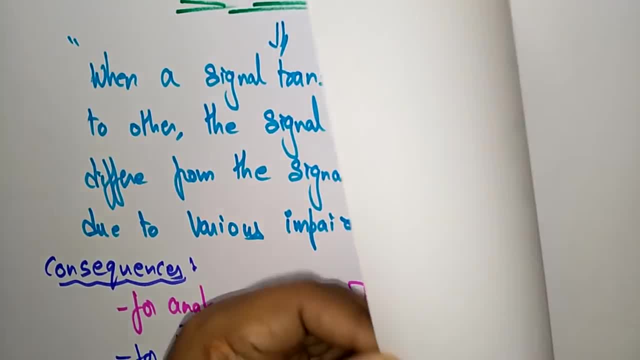 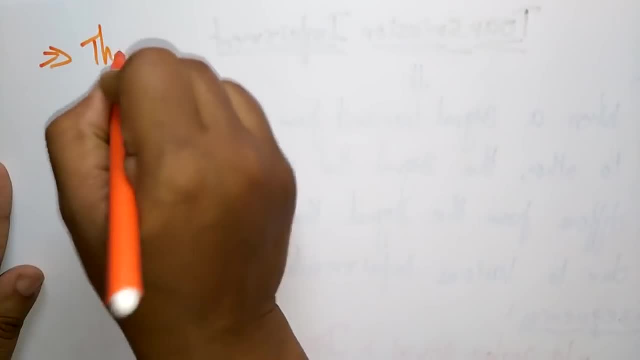 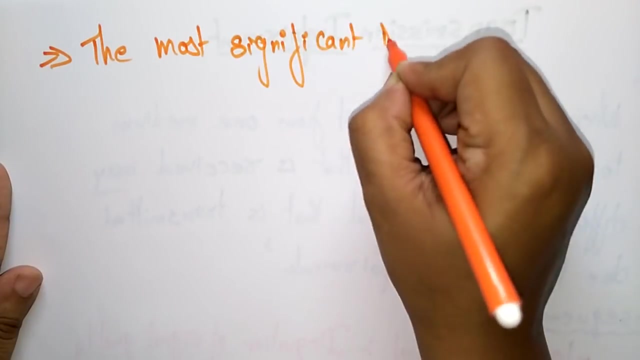 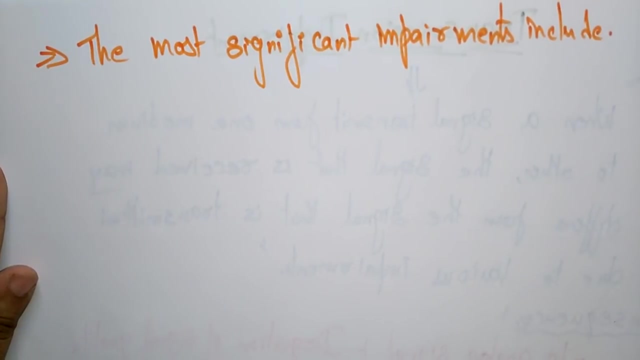 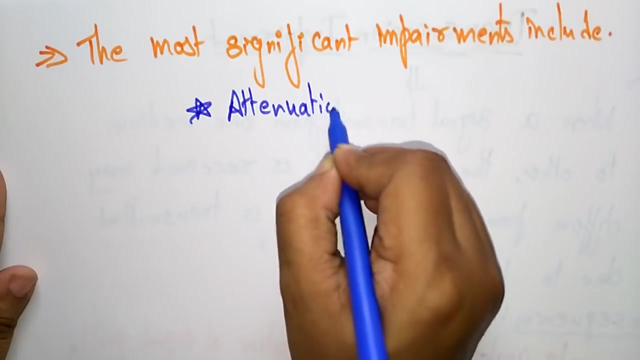 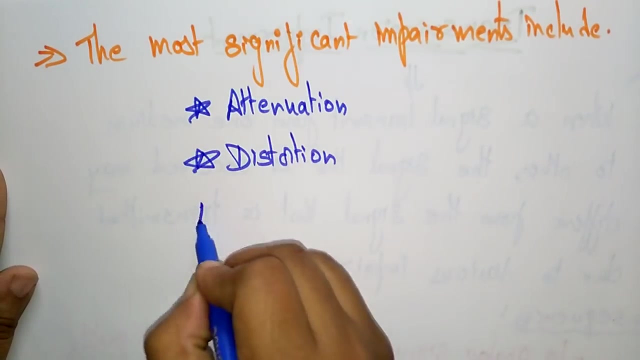 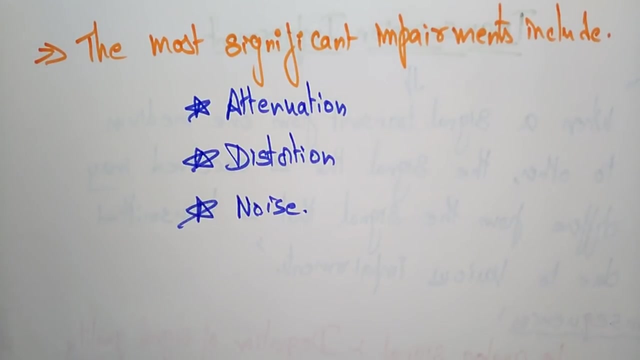 the most significant impairments include: so, whether you can take the analog signal or a digital signal, the most significant impairments include: the most significant impairment impairment: what it includes. it includes attenuation, attenuation distortion, distortion and noise digital signal. next try to write. the significant impairments includes attenuation, distortion and. 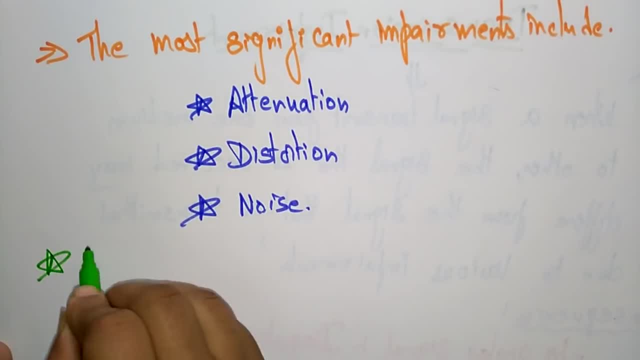 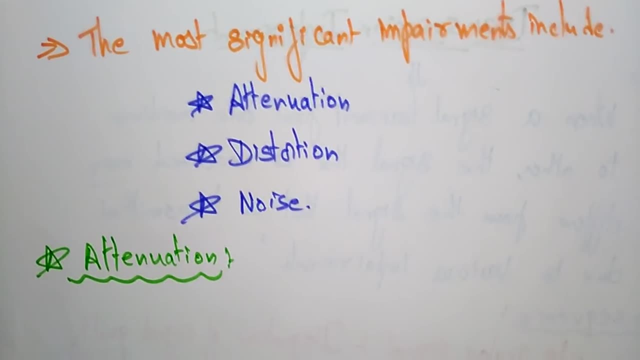 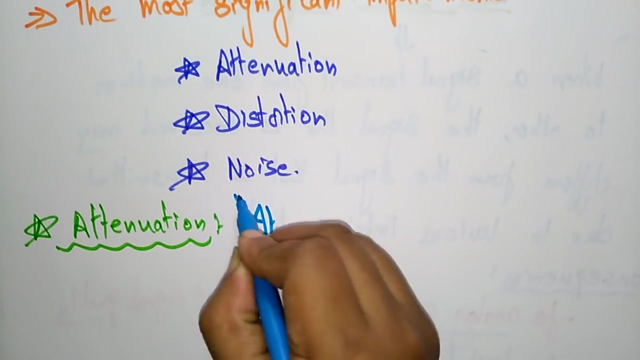 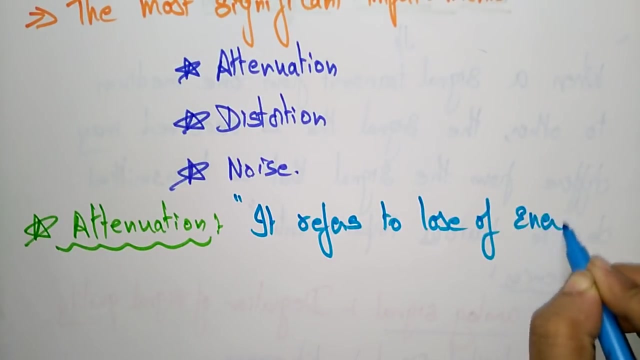 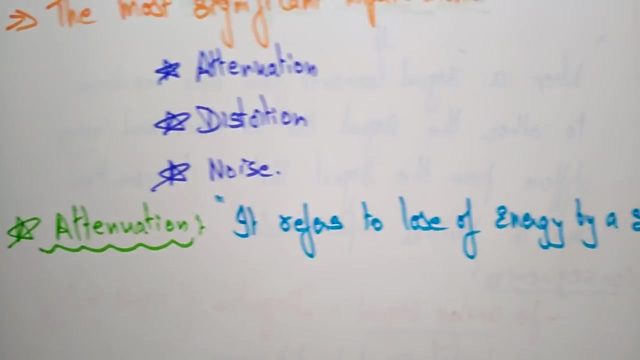 noise. let us discuss one by one. the first one is the attenuation. what is this attenuation? attenuation, it refers to the loss of energy by the signal time. it refers to loss of energy by a signal time that you call it as attenuation. so when a signal or a 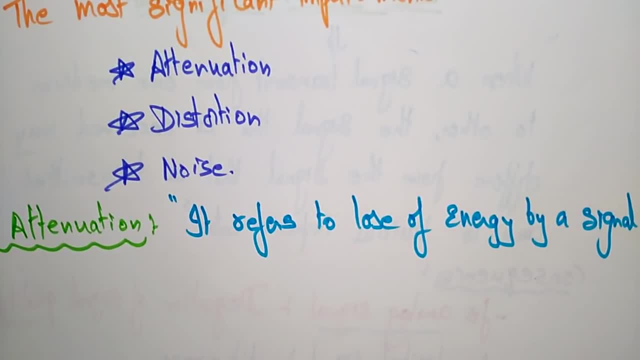 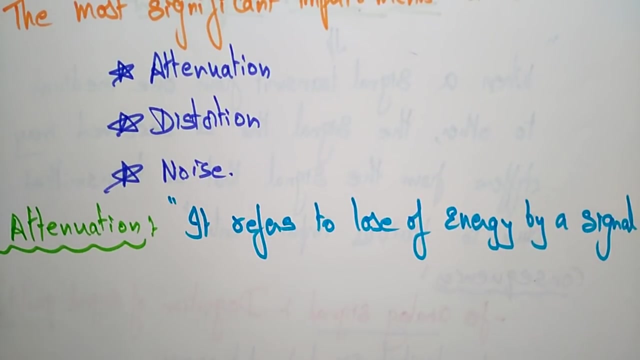 simple or it. whether it is a simple or a composite, it travels through a media. it losses some of its energy in overcoming the resistance of the medium, so it compensate for this loss of energy loss. amplifiers are used if you want to compensate this. attenuation means the loss of energy by a. 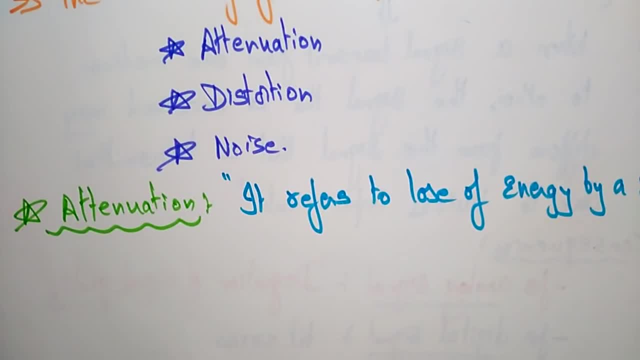 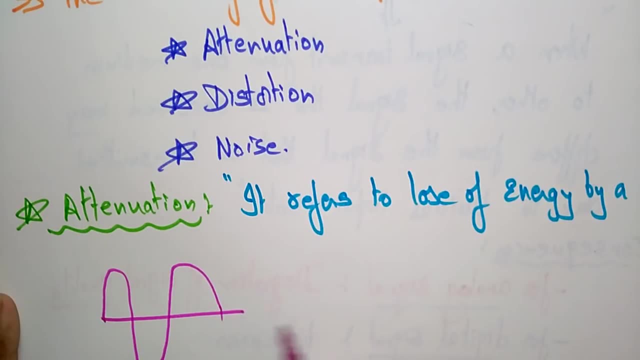 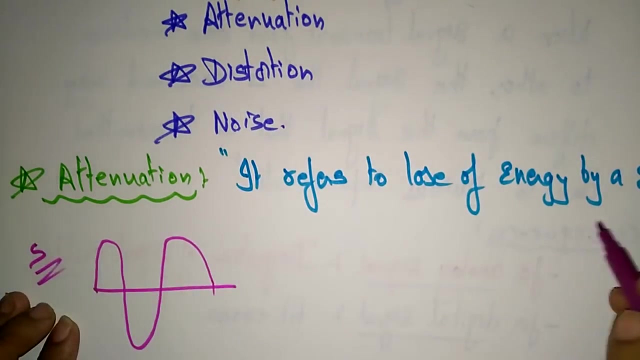 signal time, we will use the amplifiers. let me show in the form of time. suppose this is a wave, say analog signal you are, you want to transmit? okay, so this is the exact information. whatever i want to send, here the sender is there and here the receiver is there. so, while transmitting from 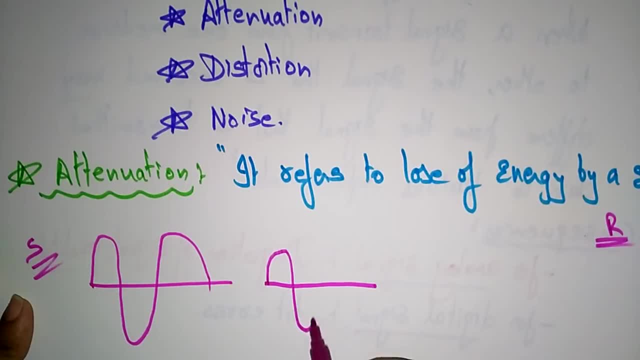 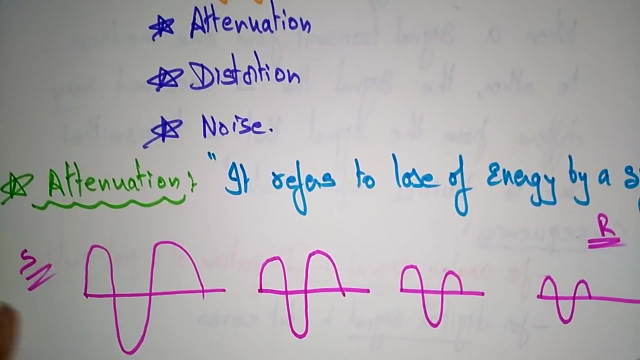 sender to receiver. the signal is transmitted from the receiver to the receiver. the signal may be somewhat: uh, loss its energy. so like this: it is losing its energy. so at the time of the receiver, the signal may be like this: this is attenuation problem. the transmission impairments, whatever the 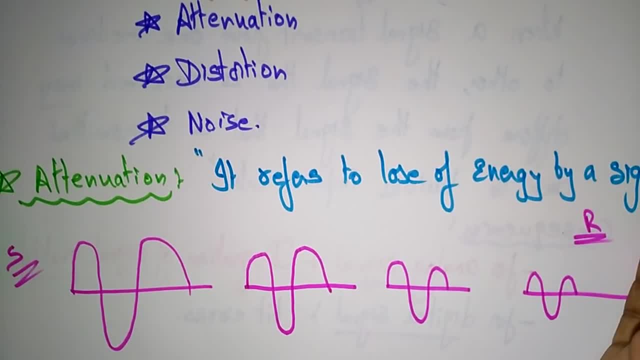 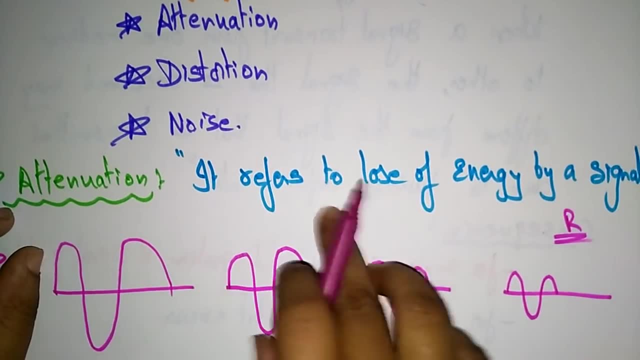 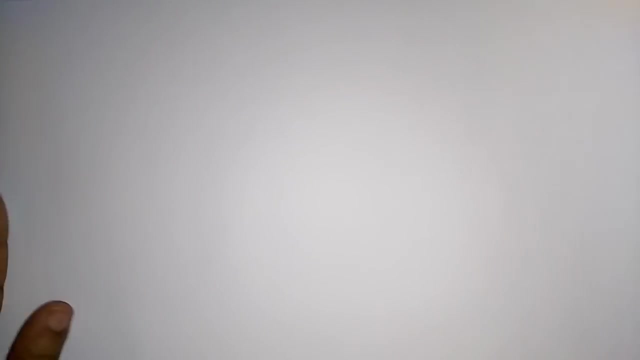 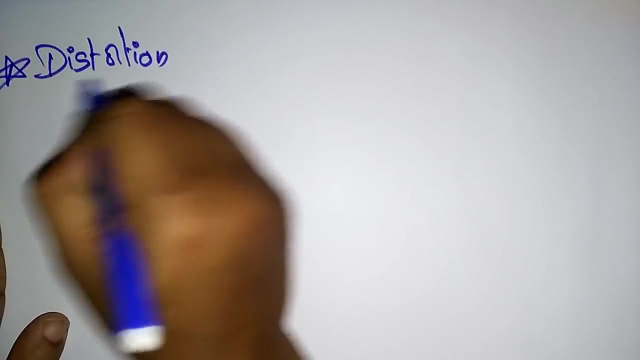 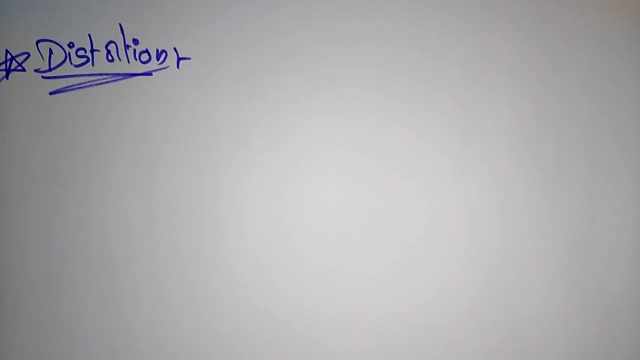 sender is sending, the receiver will not receive the exact information. so here the the most significant impairment includes one is the attenuation. it's nothing, but it refers to loss of energy by the signal. then what about the distortion? let me show you what is a distortion: distortion- distortion means signal changes its form or a shape. so here the whatever the signal. 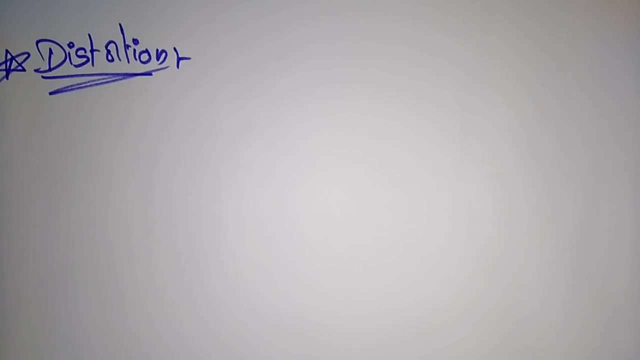 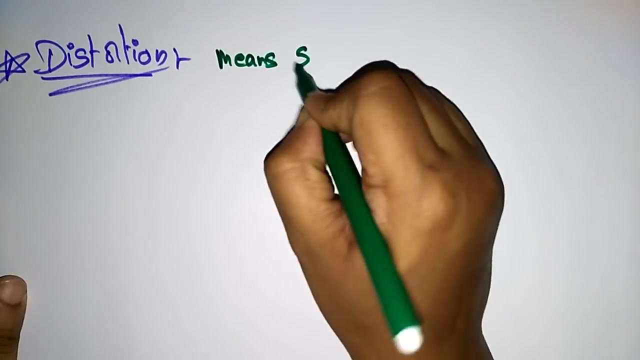 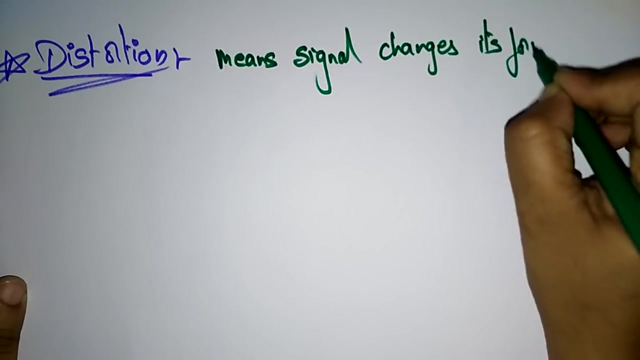 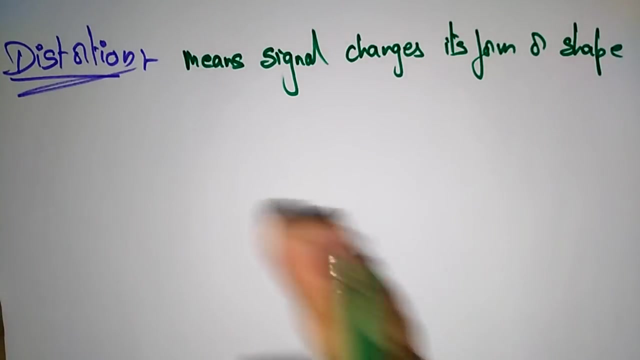 we are sending completely changing the shape. whereas attenuation means loss of energy by signal time, then distortion means signal changes, its form or even shape. also, the shape is also going to be changed, so it can occur in a composite signals made of different frequencies, whereas attenuation may be occur in 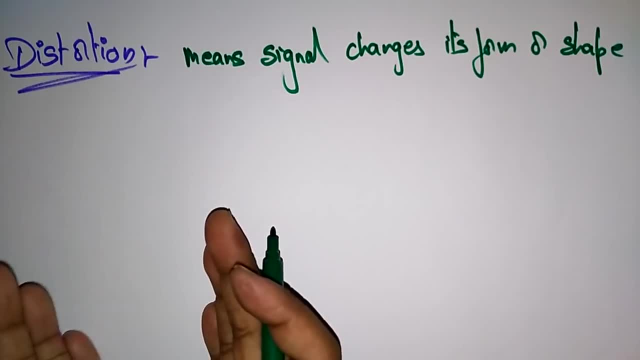 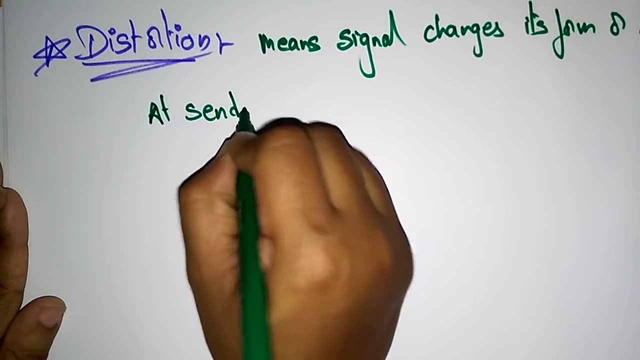 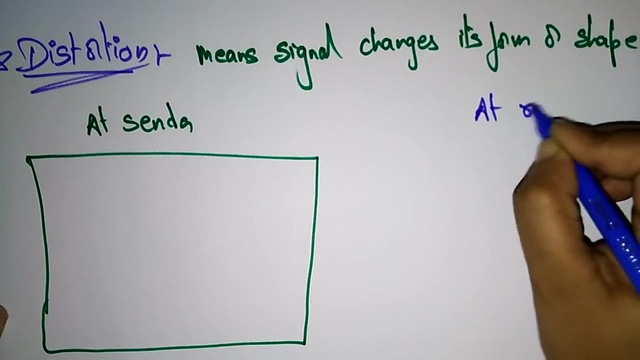 the simple or a composite, where, uh, whereas distortion is, it can occur in a composite signal made of different frequencies. let me show you: here is a sender at sender, what is going to be happen, okay, and here you just see, at receiver side, what's what the receiver is receiving. 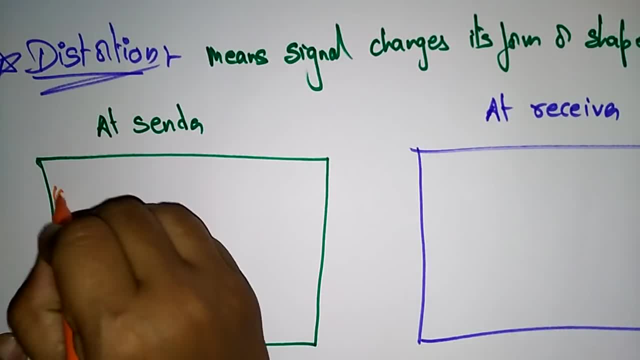 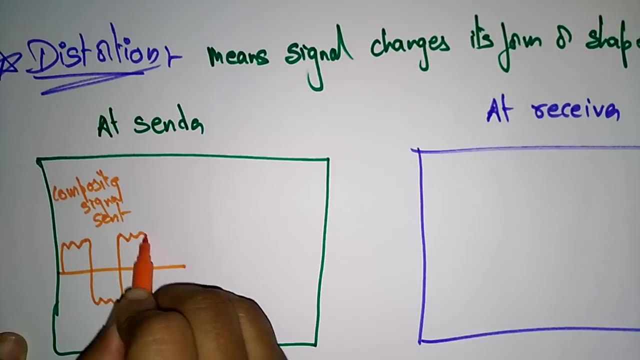 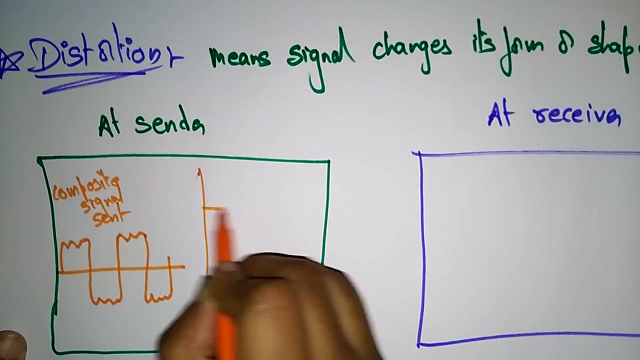 so it's completely on composite signal. i'm sending one composite signal. okay, let us take the signal was like this: so this is a signalized neat sign. let's remove that. means the data is splitting into number of bits like this. so this component is a signalized nitrate signal. 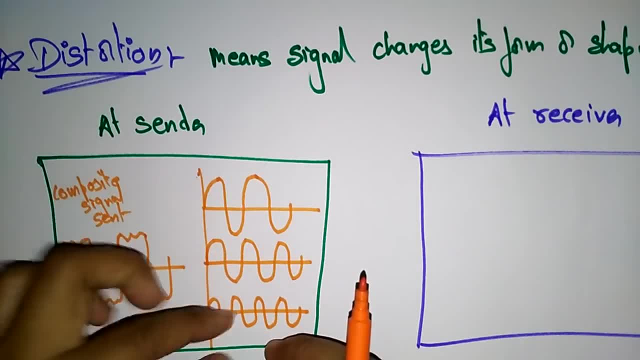 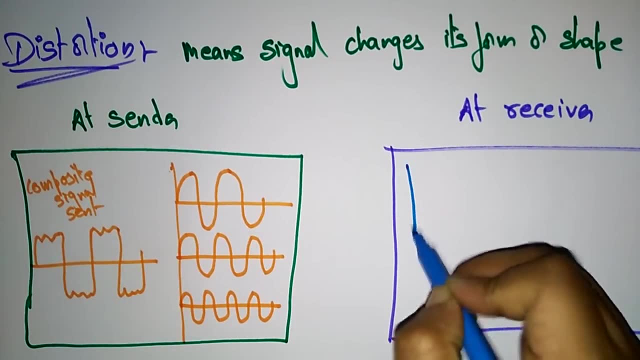 so this is the signal i signed. so this composite signal will be divided into. uh means the data is splitting into number of bits, like this. this components are in phases. now what about the? what exactly the receiver is going to be receiving? so the first: the components out of phase. so this is the 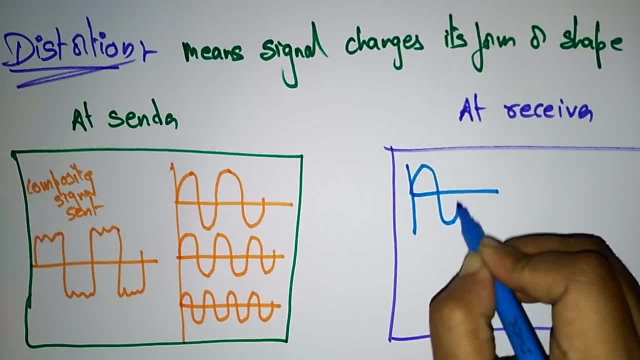 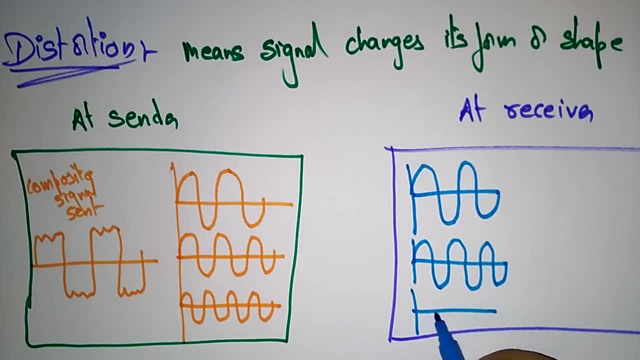 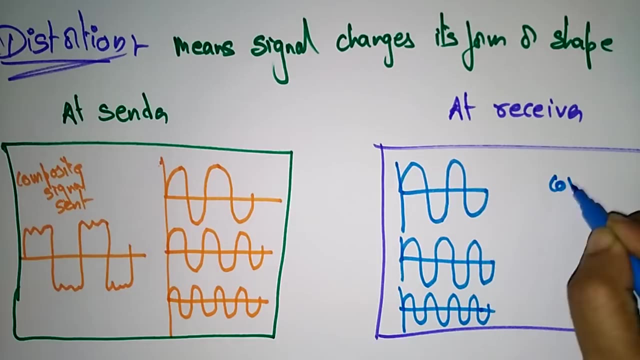 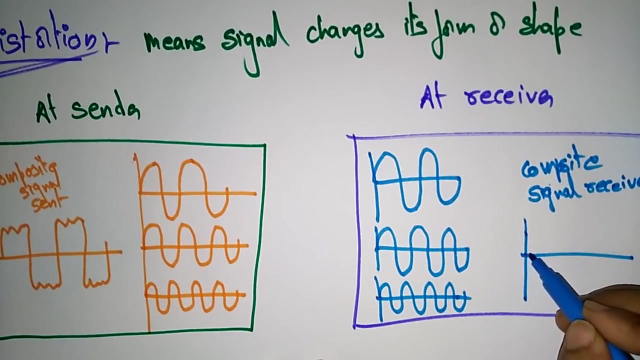 in phase and this is out of phase. up to here, it is okay. it, whatever I am sending, it is receiving the composite, the components out of phase and here the composite signal received. what is the composite signal? it is received. let's see, it's changing its shape, okay. 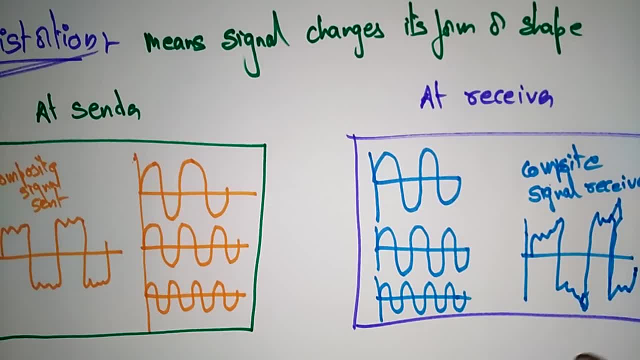 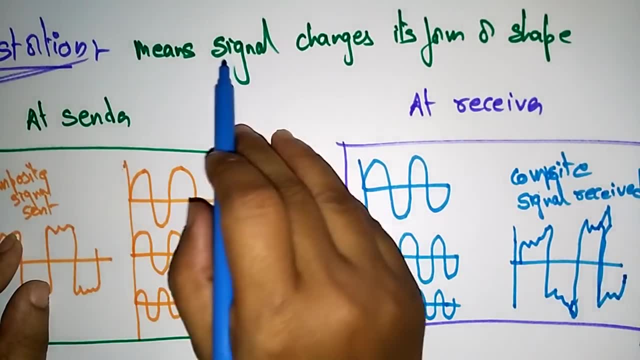 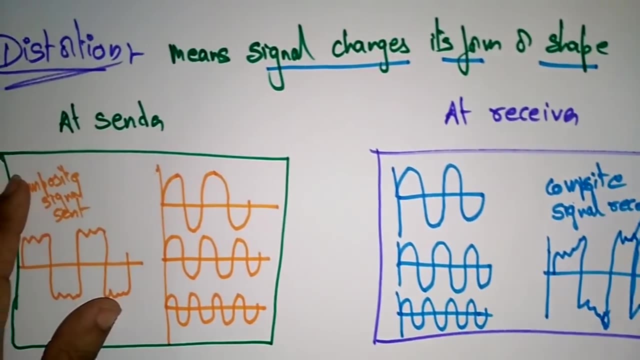 it's changing its shape. okay, it's completely changing its shape. this is a distortion, this word exactly I said, and this is the receiver is receiving. it is. distortion means signal changes its form or even its shape also. then what about the noise? the noise is a type of it's a several types of noises you can take. there are different types. 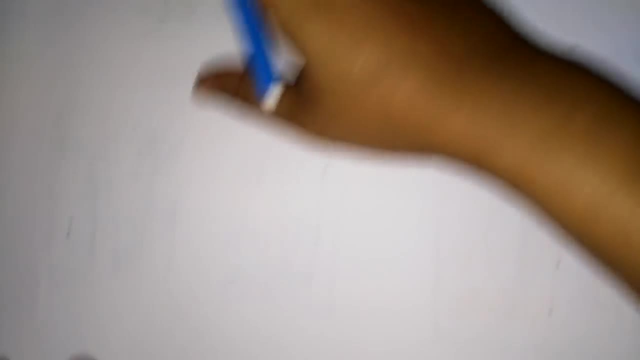 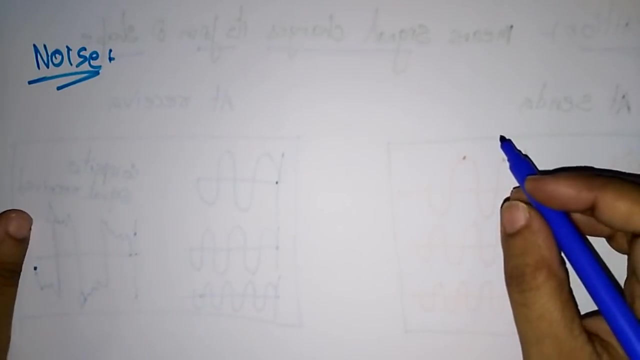 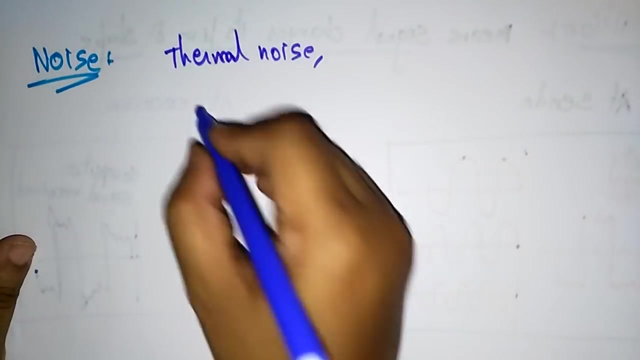 of noises will be presented. if you talk about that, noises, see also there are several types of noises. that is dermal noise, dermal noise in juice, noise in your noise or not. it's kind of noise itThat is the first one. it seemed very pleasant to me with the